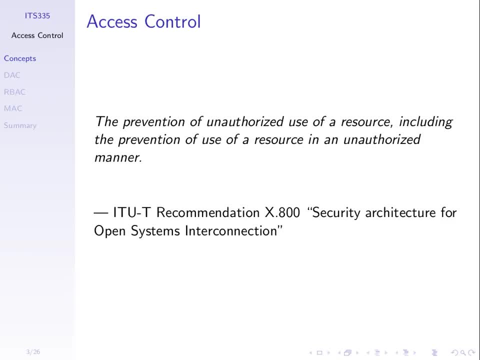 We can think that piece of software executing is a resource Memory in some cases, So the parts of the hard disk, the access to the CPU and the different operations that that computer system provides. So we want to control who can do what on our computer. 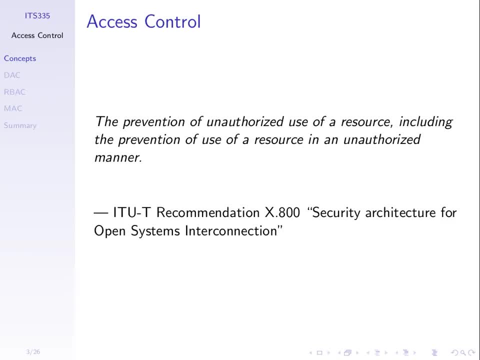 Who can access which files? Who can run which software? Who can start different peripherals on the computer? Who can start and open the CD? Who can access any other devices attached to the computer? So by resource it can be not just files, it can be physical resources as well. 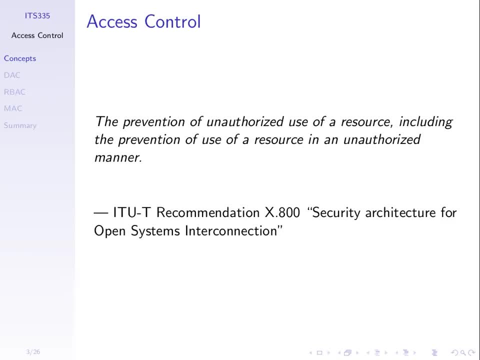 In many of the examples, I'll refer to files, because they are commonly the resource that we want to control, but there are others as well. Any questions? We're only on the definition, but there's still a lot of talking Suggest. it's a bit confusing. 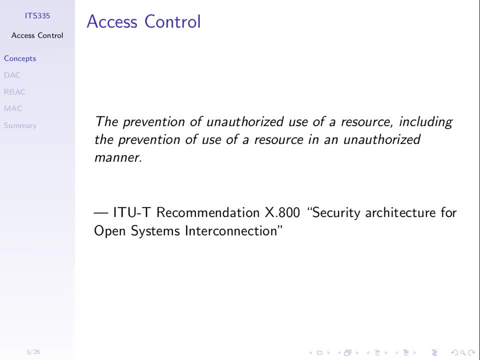 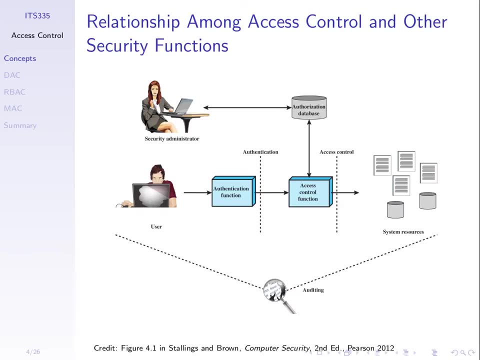 Confusing. Okay, All right, With respect to what we've seen in authentication, access control is another function involved in our computer system. So we can think, in our computer system We have a set of resources, files, databases, memory, portions of memory and so on. 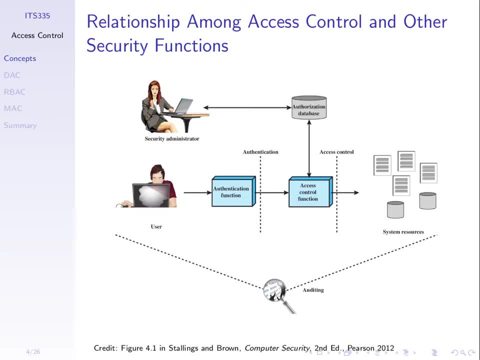 So to control which users can access them and do different things with those resources, well, first we need authentication of the user. That's what our previous topic was about saying. how can we check that this person is an authentic person with respect to our computer system? 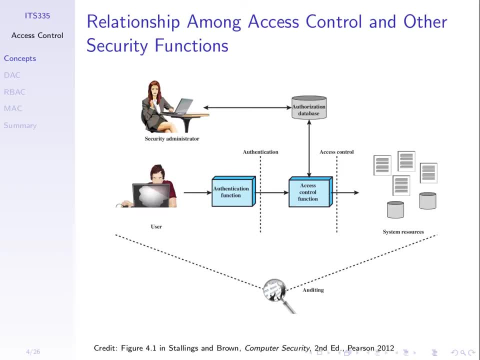 Okay That they have already been registered and that they are who they say they are. So we've looked at means of authentication. Once a user is authenticated- for example they log in- then we have an access control function to say what this user can do with respect to our resources. 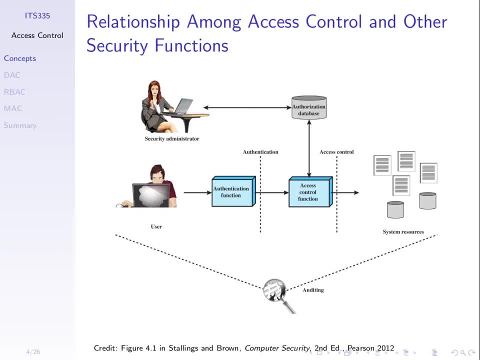 So once someone logs in, the access control function may say that this logged in person. this user with this user ID can access these resources, And we'll talk about what we mean by access shortly. So for access control to work, we of course need some authentication first. 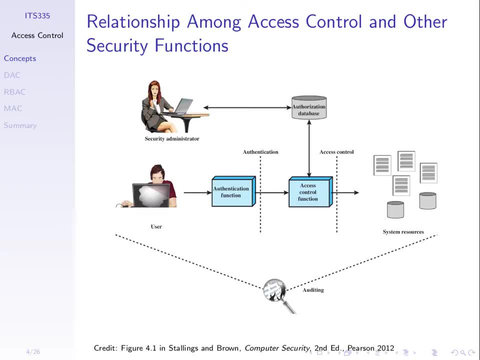 We need to make sure the users are who they say they are, Because most access control functions depend upon the user ID. Okay, That is, we say this user can do these things, So we need to make sure that we've got the right user. 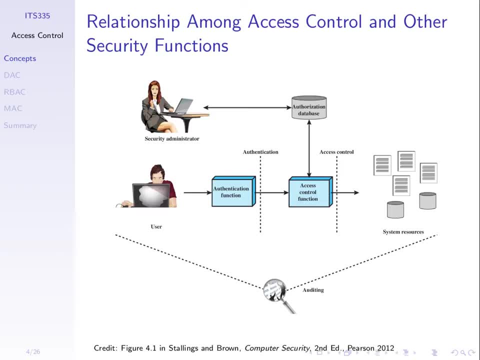 And the access control function will do things like, say, this user can access these resources, And it will control and make sure that the appropriate user can access the appropriate resources. To do so, there needs to be some database that says who is authorized to do what. 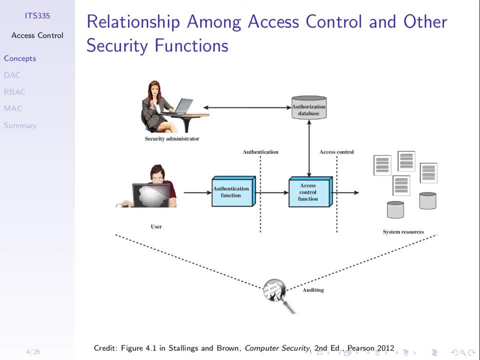 So some authorization database that says these users are authorized to access these files, For example. Who sets that up? Whoever is managing the computer system Here in the picture, some security administrator? So someone sets up the authorization saying which users can do which things. 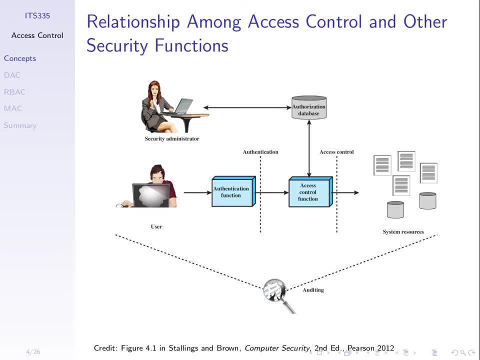 The access control function is a software that checks, based upon the user that's authenticated and logged in, And controls and makes sure that the authorizations are implemented correctly, That is, the user can access the right resources. So we've got different components all coming together now. 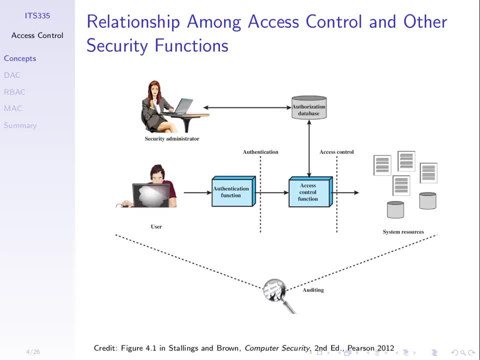 And last thing, We want to make sure that all of this works. So let's say we have an authentication system and an access control function. that controls Say that the students can only access a subset of the files on our server. So the administrator of the server has set up a database saying that these are the students. 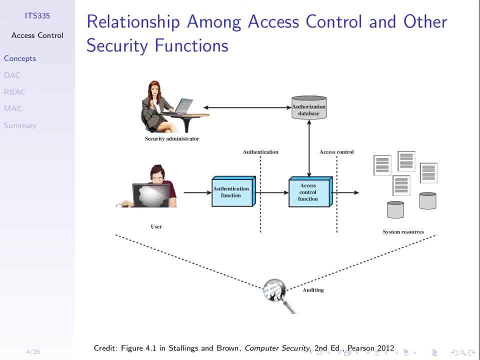 In our computer system. These are the files that they can and cannot access. Auditing is the process of checking that all of that is working as intended, To confirm that the access control is working, That the database is correct. So auditing is checking that, once we've set things up, that it's working as intended. 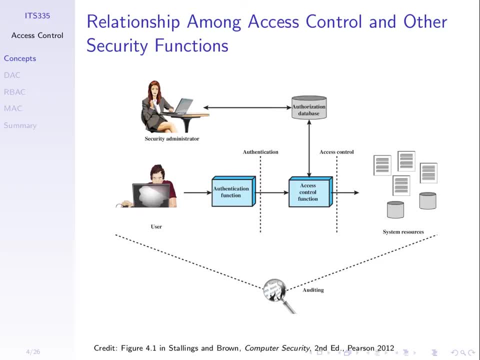 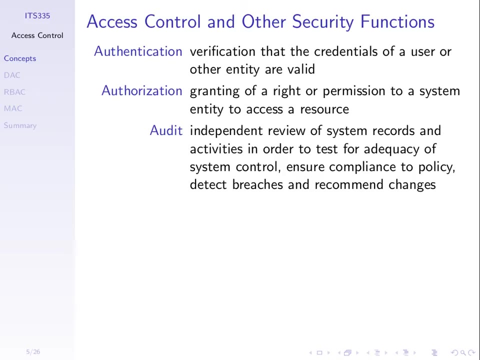 So overall we need- We're going to focus on access control, But for that to work we need authentication And also to check that it's working correctly. we also have auditing. So the other functions in addition to access control we need is authentication. 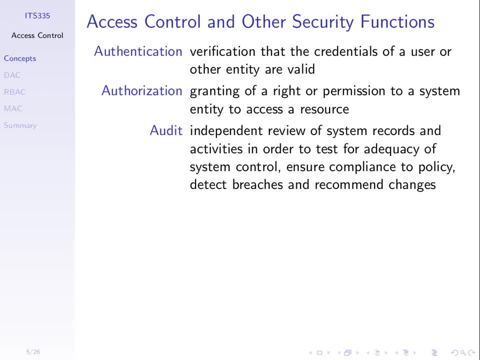 Check the credentials of the user that's trying to access the system. That's the previous topic, Authorization. So someone needs to determine who can do what. So we grant permissions or rights to users, And when I talk about users in terms of the computer system. 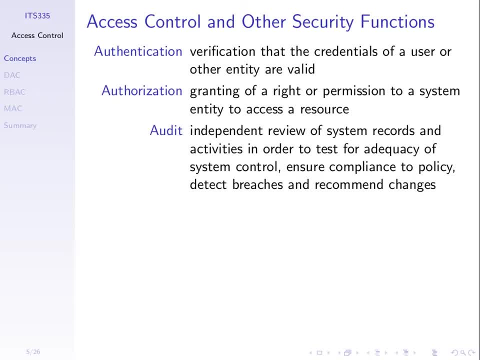 it says he is granting a right to a system entity. It may be a piece of software. I say that this software can access this file And that software may be running on behalf of a human user. And auditing is some review of the system to make sure that it's working as intended. 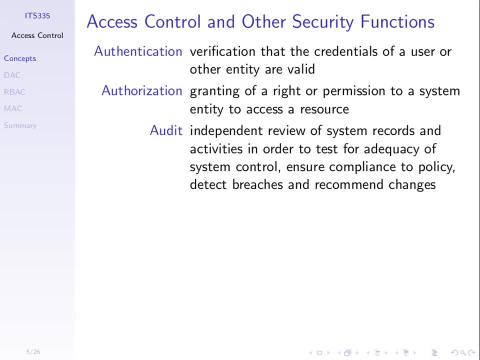 So checking that the controls are working correctly, That if we have some policy, say in our organization that says students cannot access the financial records of SIT, That may be an organizational policy. Then we need to check that our access control implements that policy correctly. 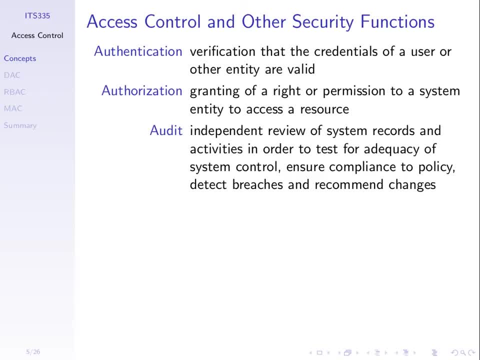 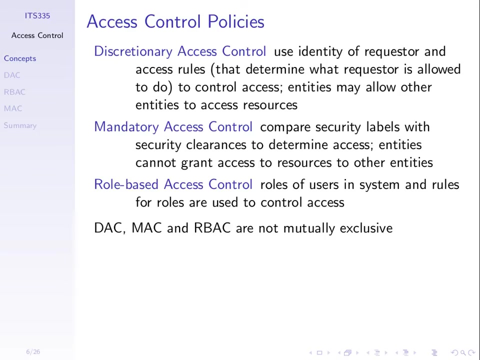 Okay And detect breaches. if something goes wrong, Then be able to detect that and fix things when things go wrong. That's the role of auditing. We're focusing on access control, The fourth one in that list. There are three main approaches to access control listed here. 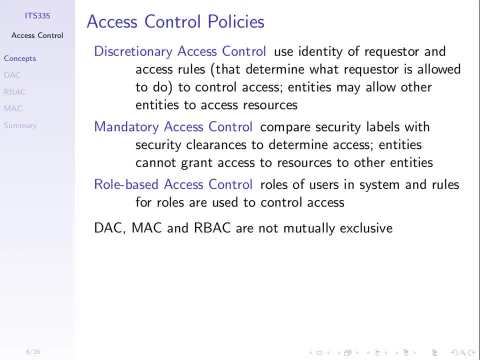 Discretionary, mandatory and role-based. We'll talk about each of them, But, as a summary, Discretionary access control is the one that we will be most familiar with already. It involves we identify who's requesting to access a resource. 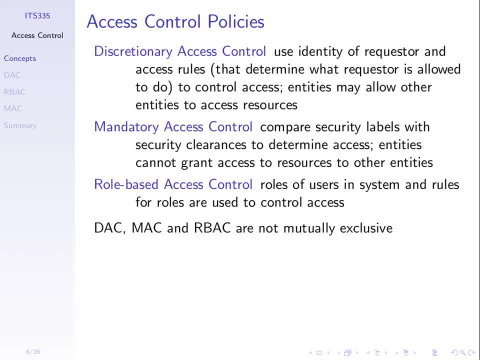 And we have some rules to say what they can do with that resource. So we need to specify those rules And it will allow entities, for example users, to modify those rules, For example to change who can access particular resources. An example may be: I can access one file on the computer system. 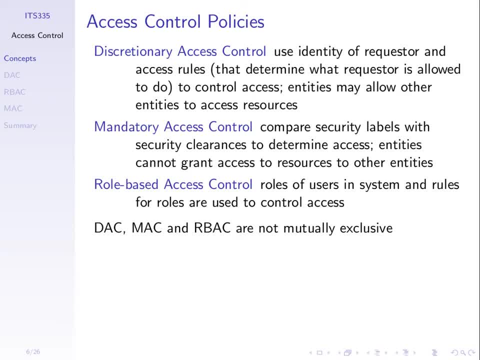 It's my file. I've created it. I may be able to change the access control so that I'll allow other users to access my file. I have the discretion to change the controls. Mandatory access control is slightly different in that we cannot change the permissions or the access controls once they've been set up. 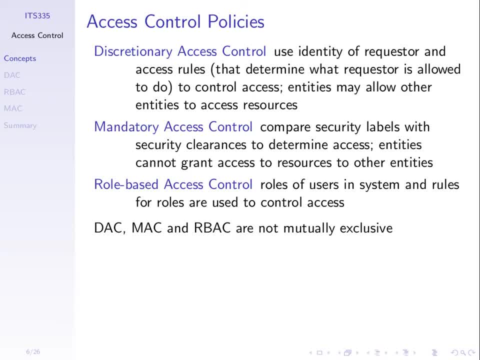 And we'll go through that And that's similar to what we'll see is security clearances, Like things in the military, are top secret, secret and confidential, And we'll talk about the relationship between different security levels and how they can be implemented in a computer system. 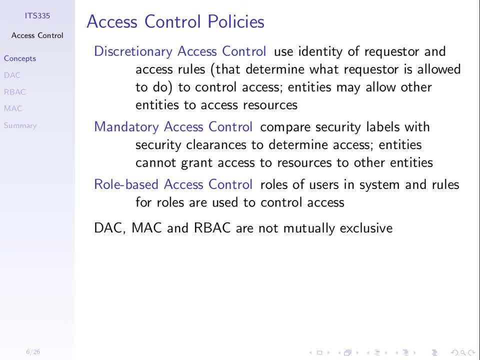 We'll see. role-based access control is similar to discretionary access control, except instead of controlling which users can access resources, we do it based upon user roles. For example, we say all faculty members. the faculty member is a role, I'm a user, but I may take a role of faculty member. 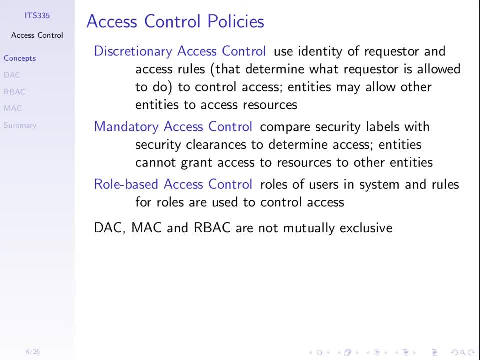 And we specify the controls per role. So I say all faculty members can do these things, All heads of school. in SIT There are multiple people who are faculty members and heads of school. They have different access permissions, So a user may take one or more roles. 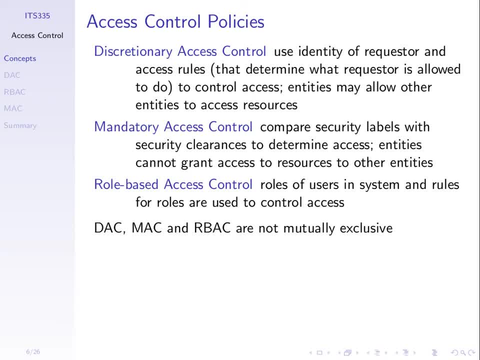 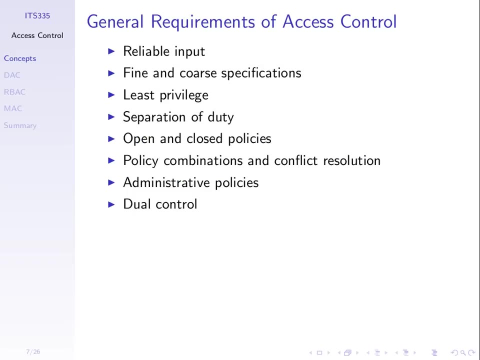 And in role-based access control. we control based on the role that they have. We can mix them So a computer system may combine these three different approaches. You don't have to use just one or the other. So let's go through them. 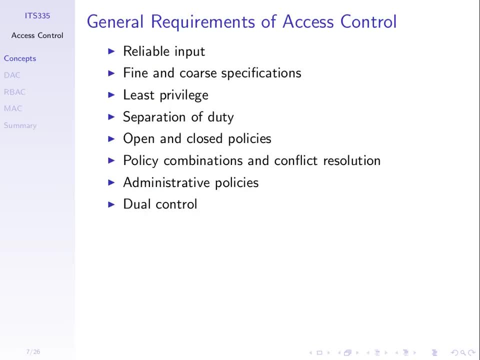 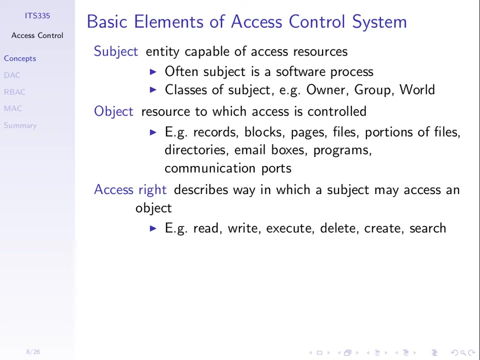 But first, I think, some basic things which are common across all of them, Actually requirements we'll return to after we go through some specifics. So we'll return to this list later. Let's go through the basic elements of access control. So all of these systems. we distinguish between a subject, an object and an access right. 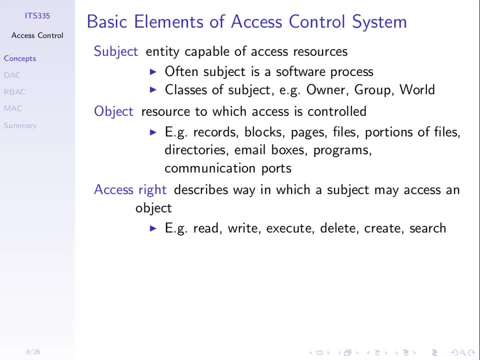 The subject is the entity trying to access a resource. Think of a person or a piece of software acting on behalf of that person. A subject wants to access some resource And that resource we refer to as an object. So the thing that we want to be able to access and control access to is we refer to as objects. 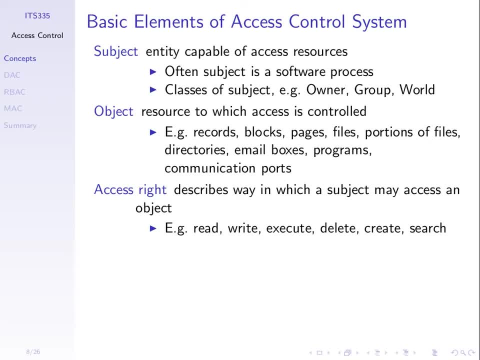 And those resources or objects may be some record in a database, Some blocks that is on the hard disk. A hard disk is split into blocks, So a particular range of blocks that they can access In memory. we can divide memory into pages, for example. 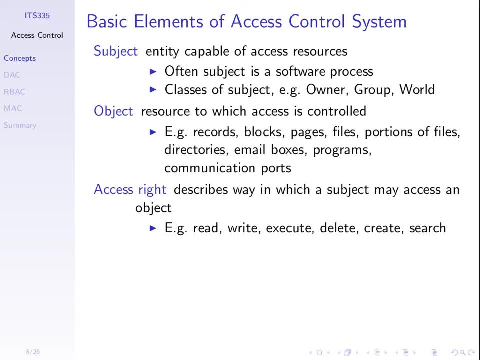 Files, So the object may be an entire file or even part of a file. So we may control very fine-grained and say that this user has access to these parts of this file, Not just the entire file. Directories, Email boxes, for example, as the inboxes for different users. 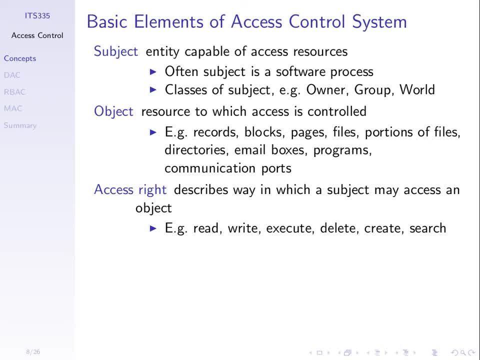 Software, so programs And communication ports or means of communication on the computer system. So there are many different types of resources, or what we'll call objects. when we talk about access control, What we want to do is specify which subject can access which objects. 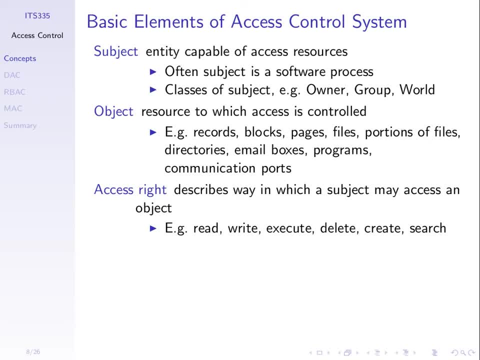 And we do so by specifying access rights, Or sometimes called permissions. We say subjects have rights to access different objects. It describes the way in which the subject can access the object. So when we say access, it may be different ways. So common ways are read: access. 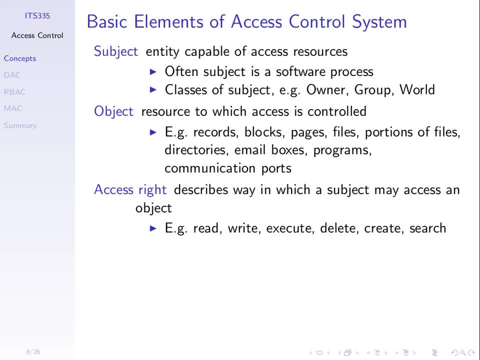 Read, for example, on a file, means you can see the contents. If I can read a file, I can see the contents of that file. Write access means I can modify the contents of that file. Execute access: The access right of execute means. 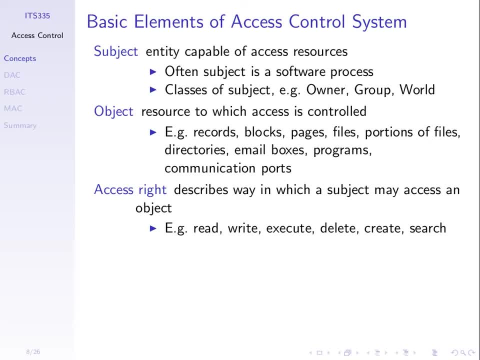 I can run that file, execute it, And there may be others, like delete. I may be able to have the specific right to be able to delete the file or not be able to delete the file. Create files, search for files. and there are even others. 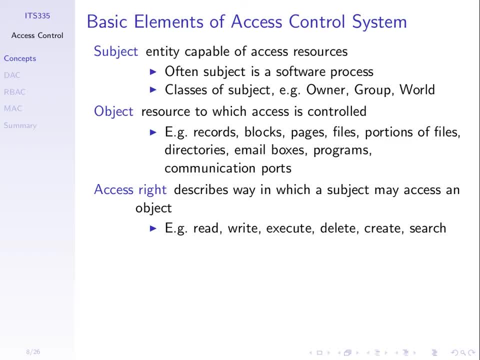 So there are different things that we may want to allow the users to do. They are called access rights. In summary, we want to specify which subjects have which access rights on which objects. For example, user Steve has the read and write permissions on file X. 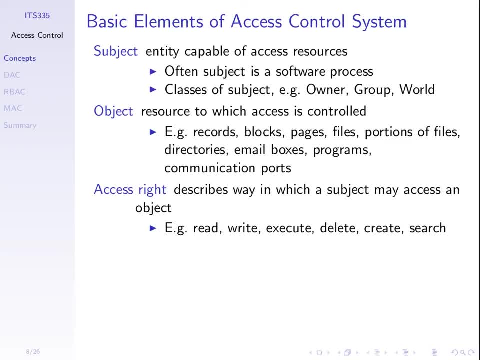 Questions on these three concepts Easy so far, And some of you may have seen these concepts in Linux file systems. If you've sat through our lab, you've seen that we've been able to give permissions to users, And that's what we're talking about here in the general concept. 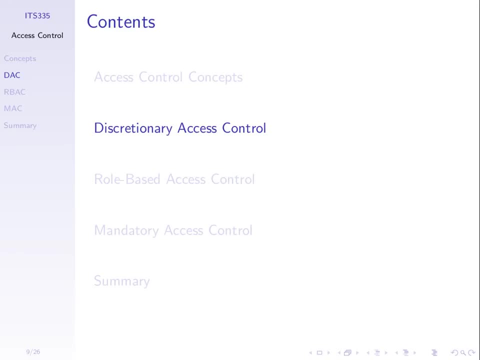 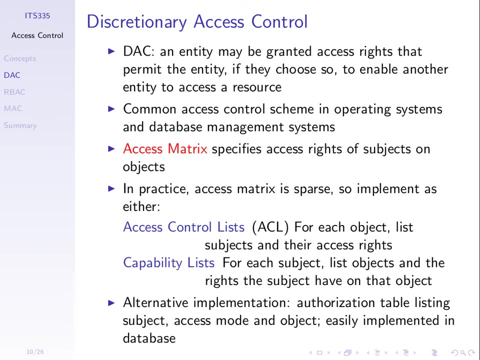 So the most common form that we'll be familiar with is discretionary access control. An entity may be granted access rights that allow that entity to enable others to access the resource. For example, I may be able to read and write to a file and I may also have the permission to give someone else permissions. 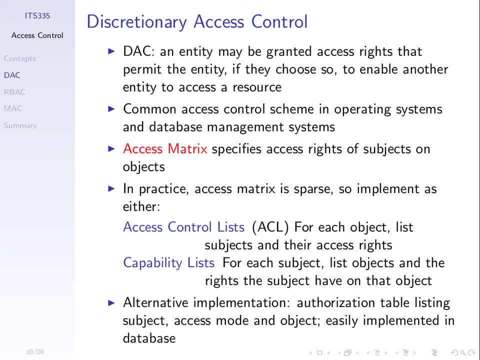 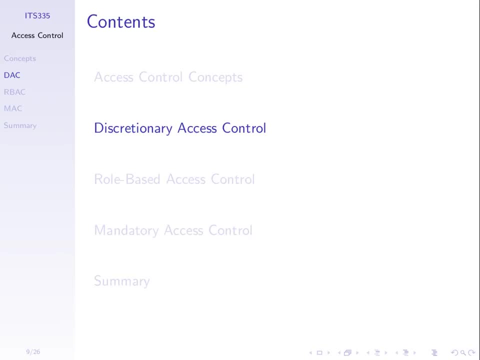 to read and write that file So we can modify the permissions or the access rights. We have the discretion to do so. That will distinguish from another type where we're not allowed to modify them once they're set up. That is just going back to our picture. 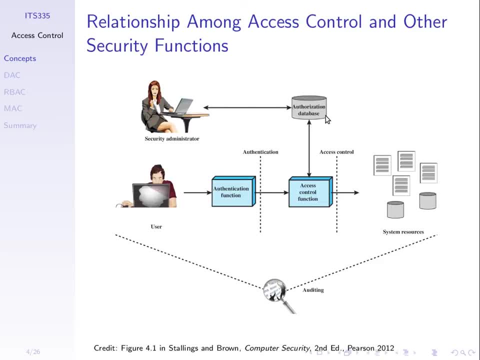 someone, initially. so there's some initial authorization database that says that these subjects have these access rights on these objects, But with discretionary access control, the users, the subjects, may change that, So they may modify those access rights as we go, Not the security administrator. 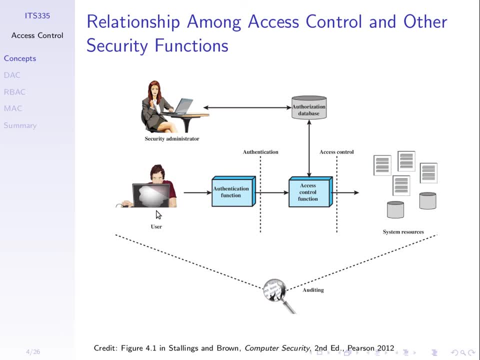 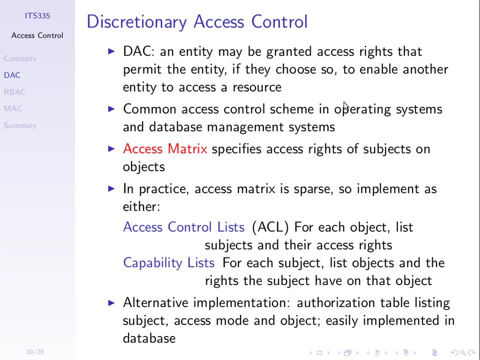 but the actual users may change the uh authorizations. It's very common in operating systems and in database management systems, which is what we're mostly familiar with. We use operating systems all the time. We need to set them up for different purposes. 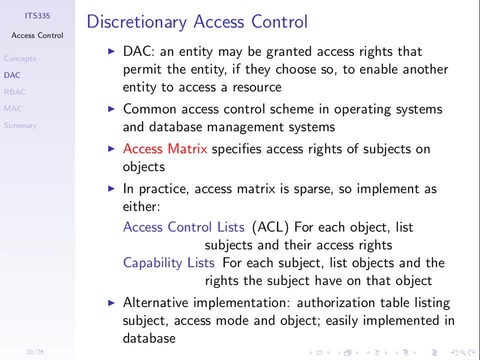 And I think some of you have- have implemented different databases or database management systems to control what users can do And, as a result, the concepts are also applied in many applications you may develop, like websites, where you have multiple users and you want to control which users can do which things. 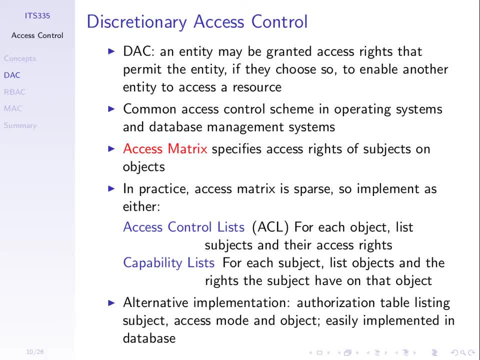 What we do with discretionary access control. we specify the access rights, we map uh for each subject, to each object on the system and we say what access rights they have. And we can think of that as a matrix, an access matrix. 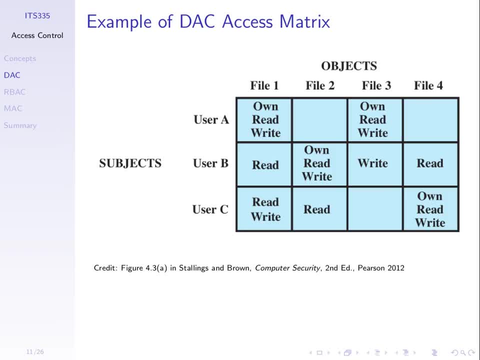 Let's go to an example, a simple example that says we have a set of three- uh three- subjects, three users on our computer system, for example A, B and C, and we have four objects. This is, of course, a trivial example. 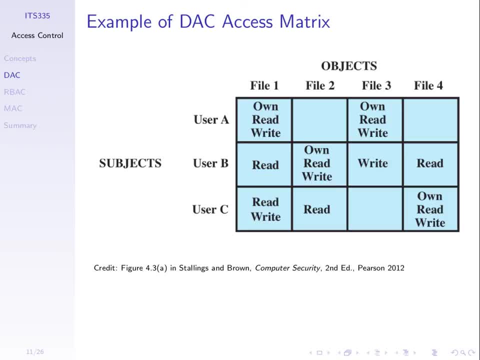 In a computer system we have uh many. we may have many more objects and may have many more subjects, But the access control can be implemented by specifying in a matrix form that of those objects. what can the subjects do? And the objects in this example are files. 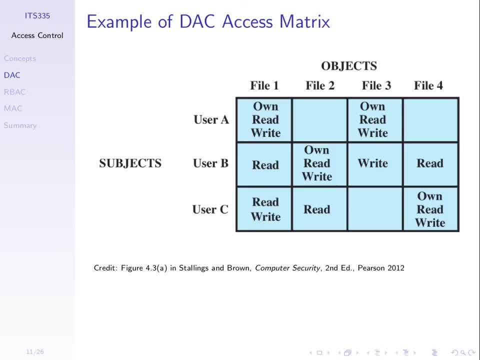 So in the element on the matrix it specifies the access rights. So subjects, objects, access rights. In this example it says user A owns the file, file 1.. So that's some access right to say that they are the owner of that file. 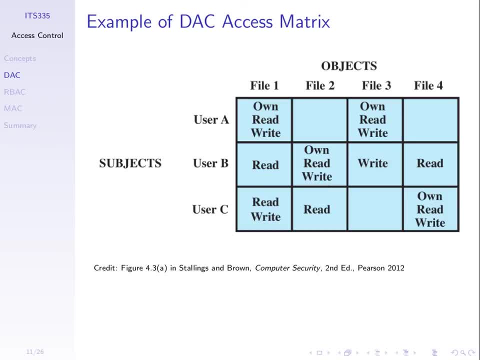 In addition, they have the right to read that file, the access right or permission to read the file and also the permission to write the file. User A has no permissions on file. 2. Being empty means that those access rights, uh, are not available. 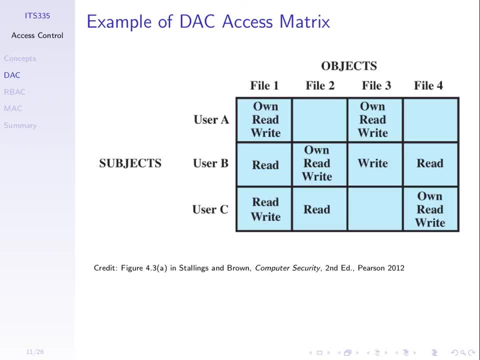 And they have own read and write on file 3 and no permissions on file 4.. And similar for user B and C. we see the access rights for this system. So this information is what's initially stored really in that authorization database. 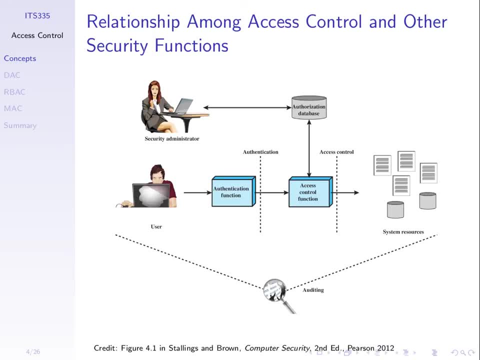 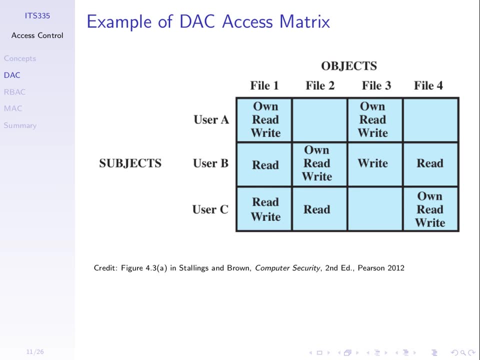 So think of the authorization database specifies which subjects can do which things with which objects, And here we're doing it as a matrix. This is just an example on files. It doesn't have to be on files, It can be again on on memory. 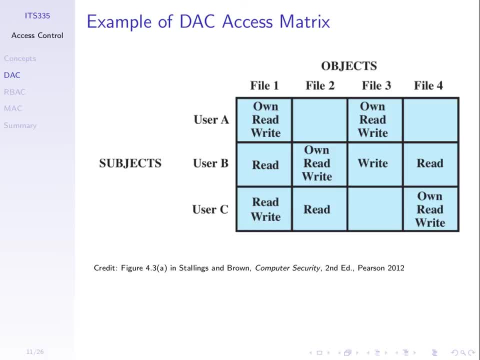 parts of files, different resources inside our computer Files, is the easiest example than the most common one we see In this example. read implies that we can see the contents of the file. Write implies that we can modify the contents, which often also means we can delete the file. 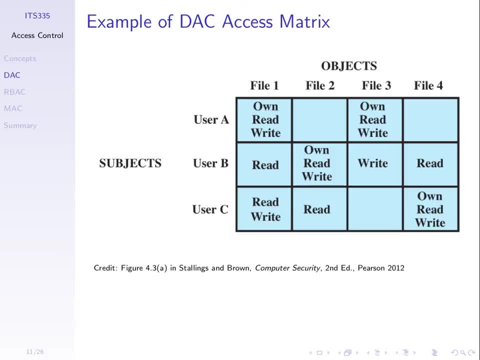 Let's say it's a text file, If I'm allowed to modify the contents and save it, one thing I could do is just delete all the characters in the file and save it as an empty file, which is almost equivalent to deleting the file. 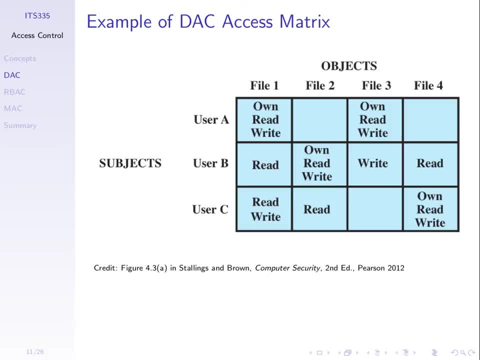 So write sometimes implies that it also means the ability to delete an object. What do you think ownership means? If I own a file as opposed to not own, what extra thing can I do? What can user A do to file 1 that user C cannot? 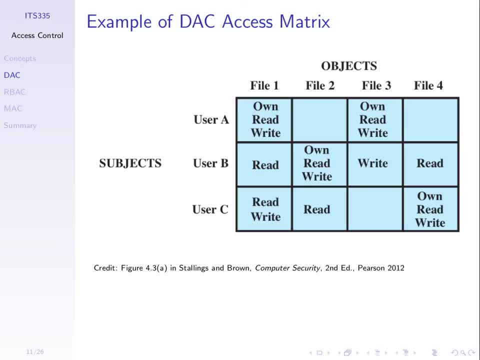 Well, if if we say that write permission means that we can think of, write means you can modify. So I open up the file as user C, I'm allowed to write the file. It says user C can write the file. 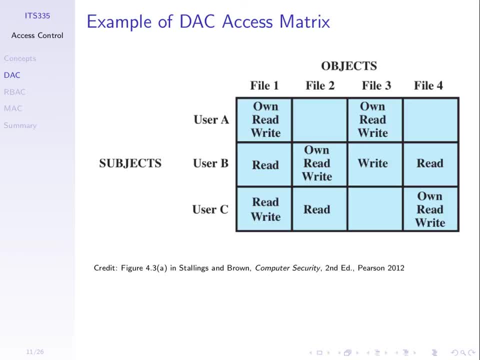 Then I open the file in my editor and I remove all the characters and save it. That's effectively deleting the file. There's nothing that's left. So no, not necessarily delete. It depends upon the, the exact implementation. Maybe there's another thing that user A can do. 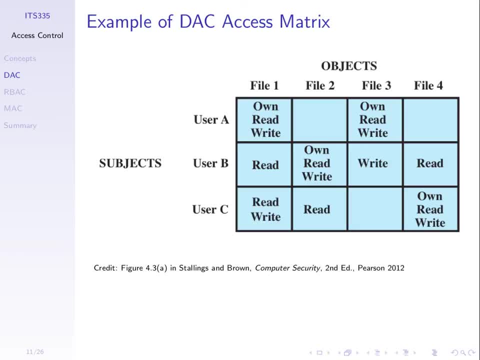 but user C cannot in discretionary access control. What do you think the own helps for? Delete and remove are about the same. But delete is fine, Right, but the contents of the file are gone. Maybe the file name is still there, but there's nothing in it. 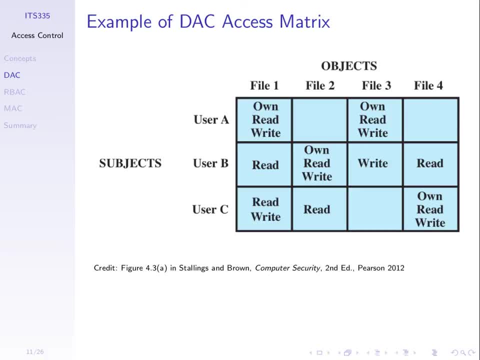 So it's effectively deleted. What else Ownership? What can that provide me? Ownership generally implies that I can right I own that file and in discretionary access control means that I have the I'm allowed to change the access rights on this file. 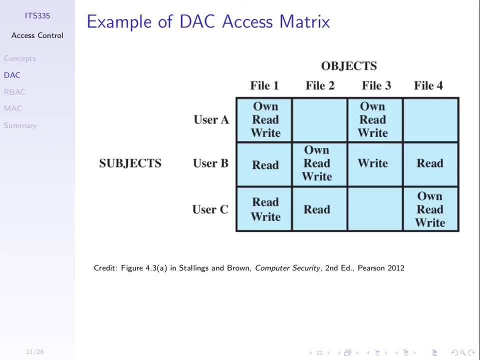 That is, I may change it for myself and, more importantly, I may change the access rights for other users, Since I own file 1, user A owns file 1, user A can allow user B to also write it, So they can modify this set of permissions. 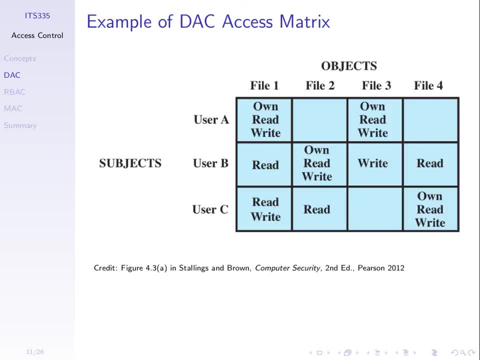 Or they could modify the permissions for user C that user C can no longer write file 1.. So in discretionary access control the users have some discretion in modifying these permissions And usually that belongs to ownership. The owner has the discretion to modify the permissions for that object. 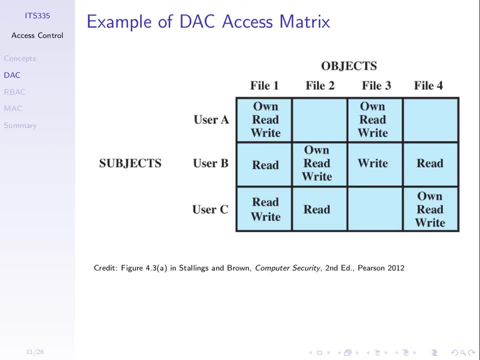 Think of your computer or a computer system that you use. that may be multiple subjects, multiple users. How many files on a computer system? Four or more, More, Many, more. Okay, So there may be many files on a computer system, and so our matrix gets quite large in this direction. 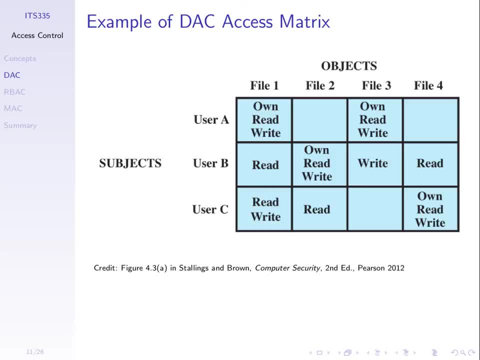 There are thousands, maybe millions of objects that we want to specify. So think of it as a matrix- becomes a bit complex because you may find that many of those files are objects. Users have no permissions, So it becomes a lot of these empty elements in here. 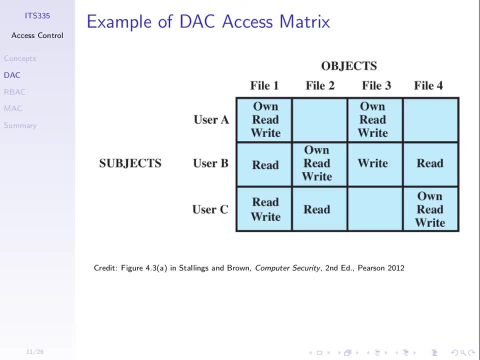 So there may be many files that one user may have permissions other users can do nothing with, which is common in practice, So that instead of thinking of it as a matrix and even implementing it as a matrix, usually we condense this information into a list. 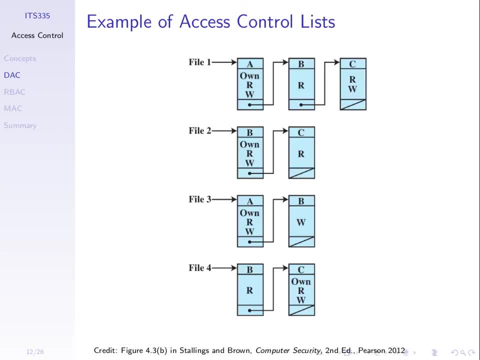 So there is what's called access control lists. This is the exact same set of permissions, but represented in a different data structure. Instead of as a matrix, we have a set of lists, And in this case there's one list for each file. 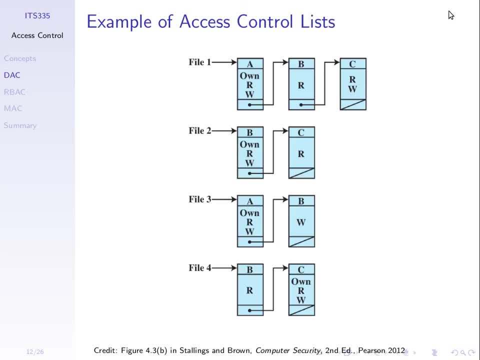 each object, File 1,. in some list or some linked list we say that user A has the permissions of own read and write, So R and W just short for read and write. User B has the read permissions and user C has the read and write permissions. 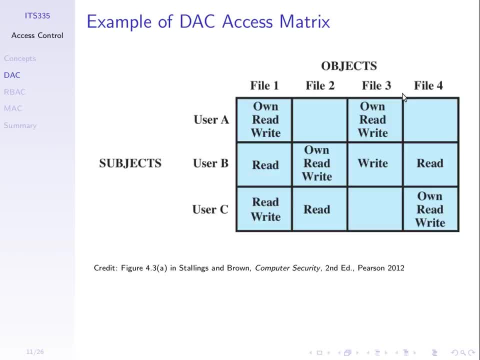 And you check. that's for file 1, that corresponds to the first column. The information in the first column is stored in that list, So it's exactly the same information. it's just a different way to store it, Because this information needs to be stored. 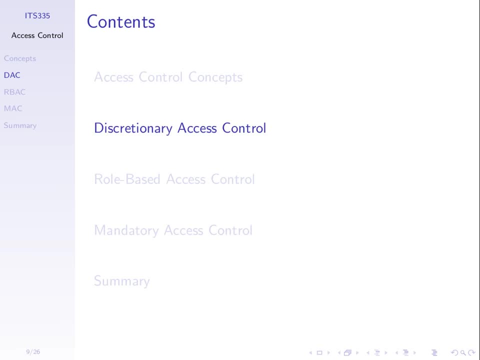 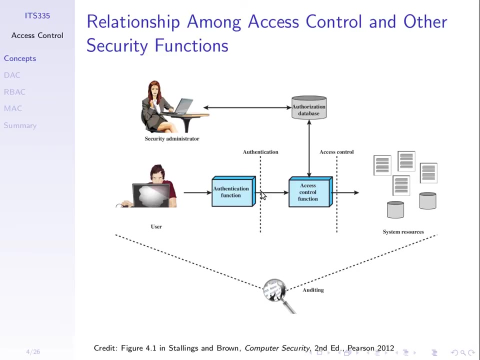 on our computer system so that think of it as this authorization database. it needs to be stored here so that when a user tries to access a file, our access control function will check that and determine if they can access it or not. So the way that we store that is actually important. 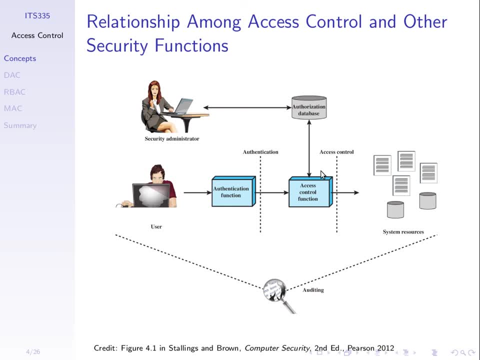 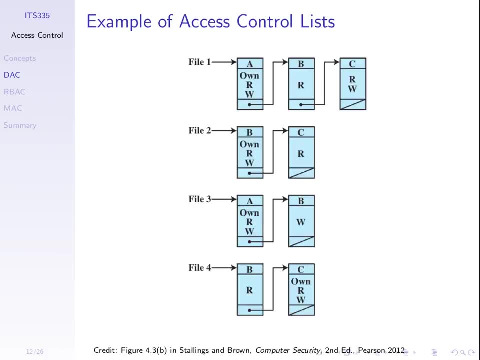 There are different approaches. So access control lists for each object in our system they specify what different users can do with that object. So for file 2, user B and C can have different permissions. User A is not in this list. 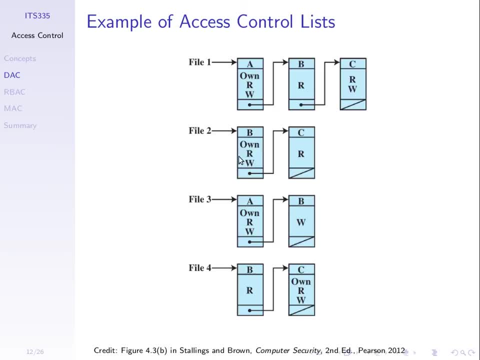 So we only list the users that have some access rights. Those that have no access rights are not listed and that saves on the storage, really, or managing that system. So if we have a thousand users in our system and only two users can access file 2,, 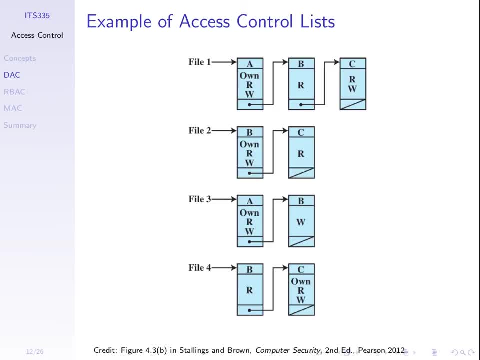 then we just have these two entries. We don't need to have entries for all the other users, because it implies that if the user is not in this list, it means they have no access rights. So it's just a more condensed way to store the information about the access rights. 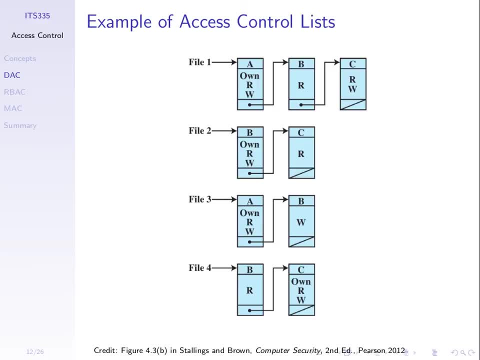 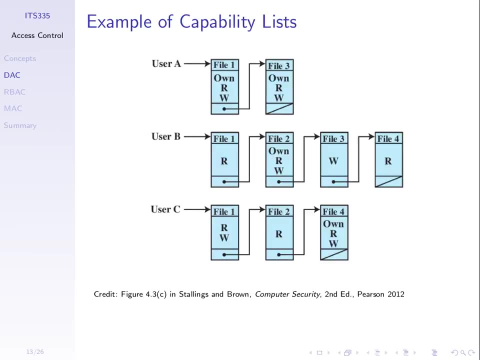 Access control lists for each object lists the permissions for each user and the alternative is a capability list For each user lists the permissions or the access rights for the different objects, what capabilities they have, And this is exactly the same as our original matrix. 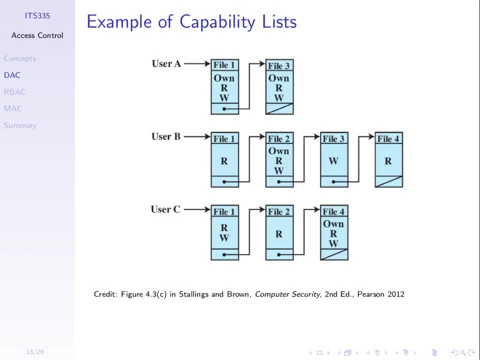 so the access control list. It's just a different data structure for storing this information. User A is allowed to well, they own file 1 and they can read and write file 1.. They also own file 3 and can read and write. 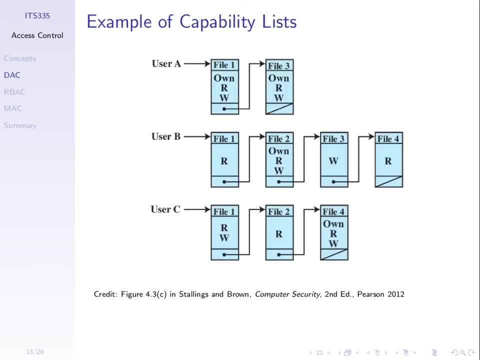 All the other files on the system. they don't have any permissions. So by this is, for example, if we have a million files on the system, then we only need to deal with, you know, entries for the files that that user. 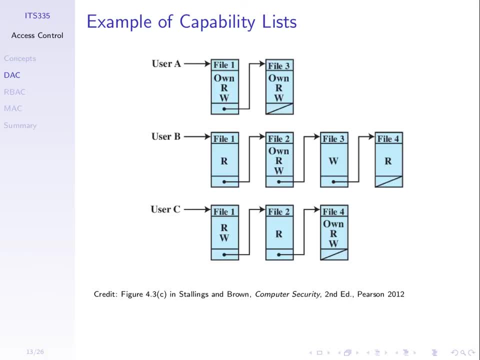 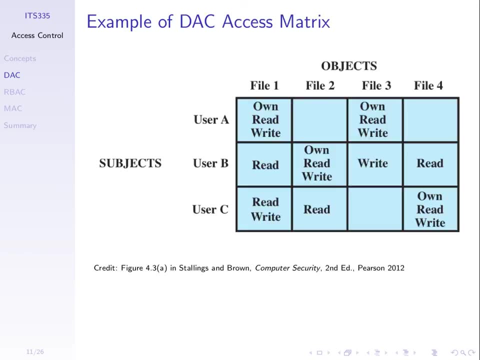 can actually do something with, We don't have to worry about others. And user B. So just check that, that the data in these three representations are the same. Okay, And if you see that, really look at the column. 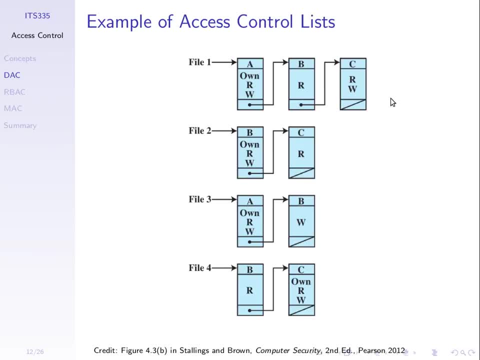 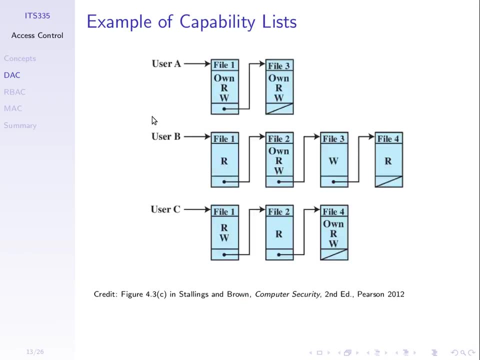 file 1, and that's the access control list. If we look at it row-wise, so user A, that's the capability list, And in fact different systems will use either usually access control list or capability list. The matrix is usually 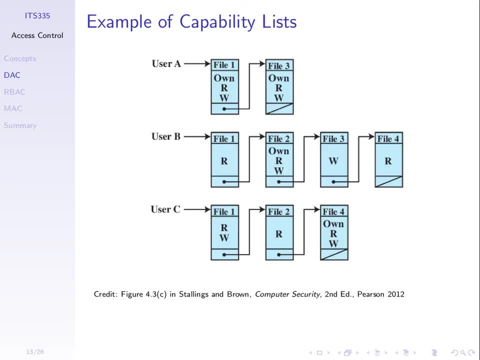 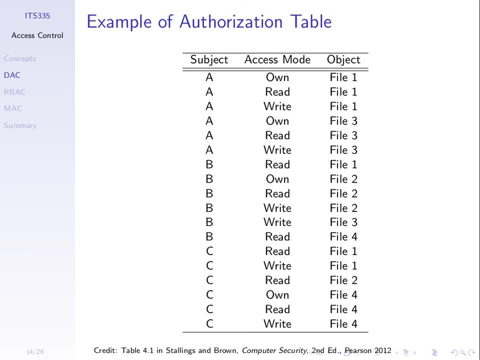 inefficient for storage and for updating. Or a fourth option, an authorization table, Simply a table saying a row for each combination of subject, object and access right Or, in this case, listed access mode. So again, same data as the previous three. 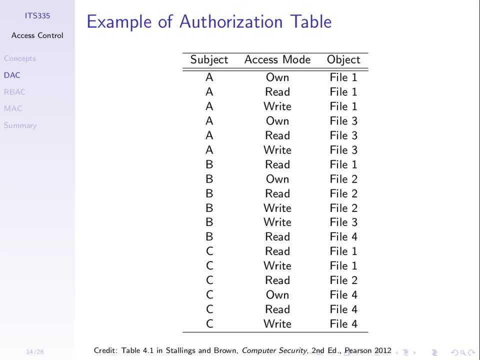 Subject A, user A has the access right of own on object file 1, and so on. So a table that has a row for each access right of combinations of subjects and objects. Here it's listed. access mode- It's just another name for access right. 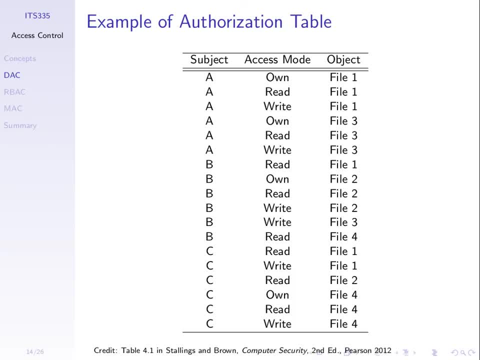 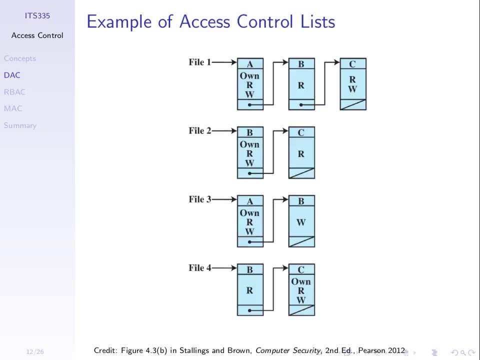 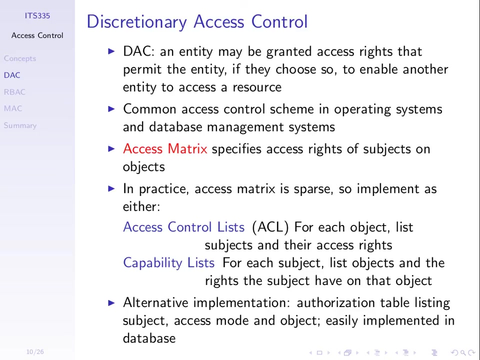 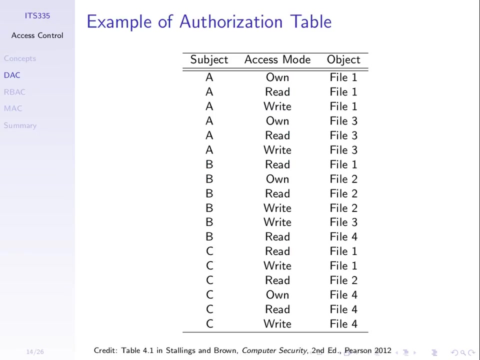 The mode at which we can access that object. Authorization table, capability lists, access control lists are commonly used in practice, but they are all just more efficient ways to store an access matrix. So they are listed there, Those three alternatives to the access matrix. 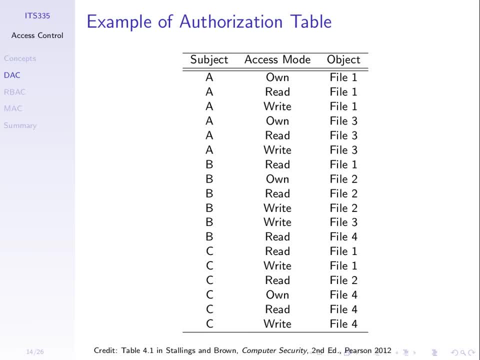 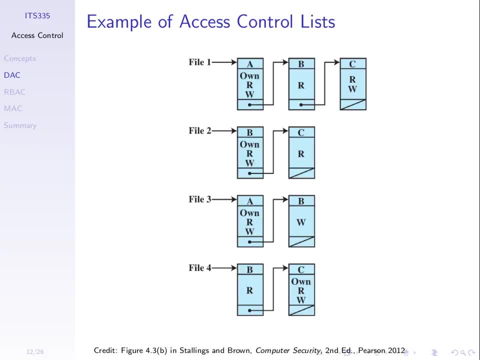 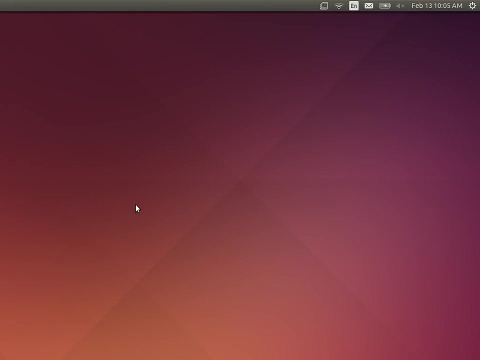 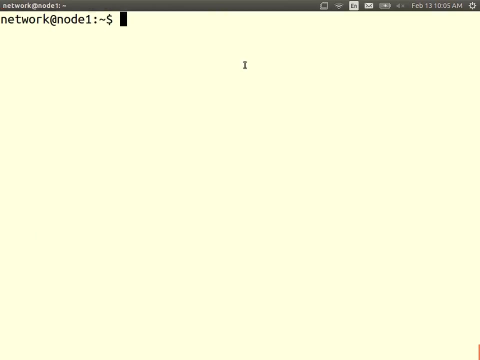 Easy so far. Let's go to an example, And I think some of you have seen the example before, but we'll spend some more time on it. Just to be clear, And the examples we'll use for access control are on our Linux operating system. 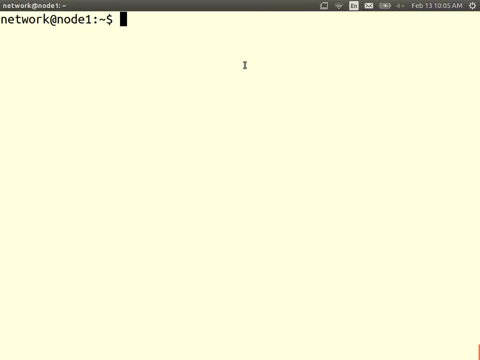 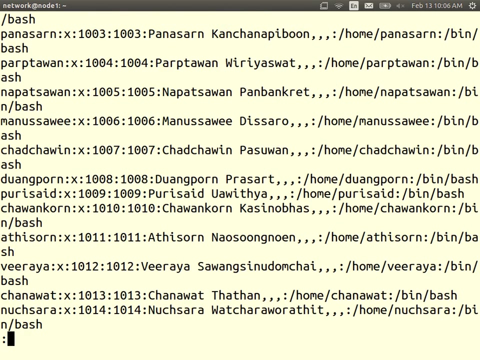 We have a set of users on this system And we saw them yesterday, but just to remind you who's there, Password is the file that stores the user information, And there are many users on this system. In fact, each of you are a user on this system. 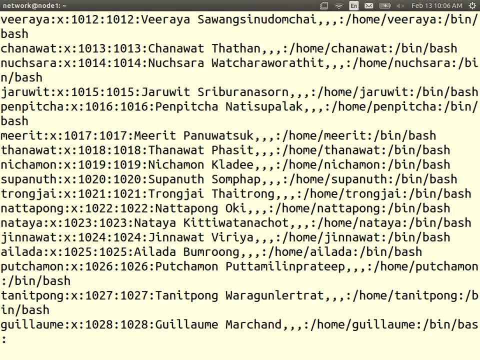 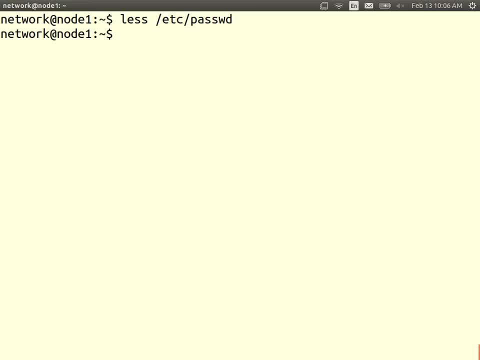 So your user names are there, And then another file in the shadow file is the password information. How is access control implemented on our Linux operating system? Where do I find out which users can access which files? How do I know? How do I know which user can access which files? 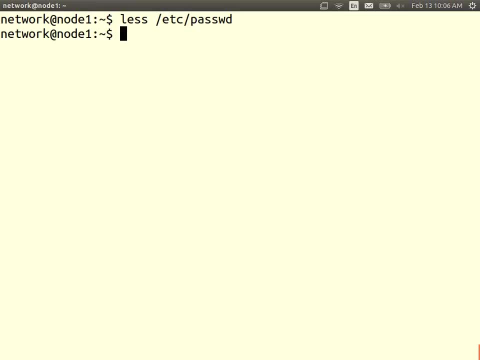 Can any user on my operating system access any file? No, There is some permissions that control what a particular user can do, And we've seen it before. We'll do it again. If I try to look at the file that stores the password information. 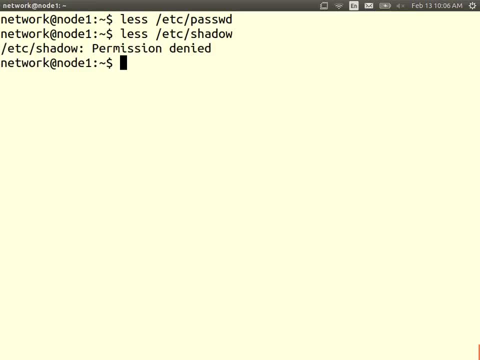 it's called shadow. It's in the etc. directory, Commission denied. That's access control working. The access control function is checking. The object is the file. Shadow is the file name. That's the object. The subject is the current logged in user. 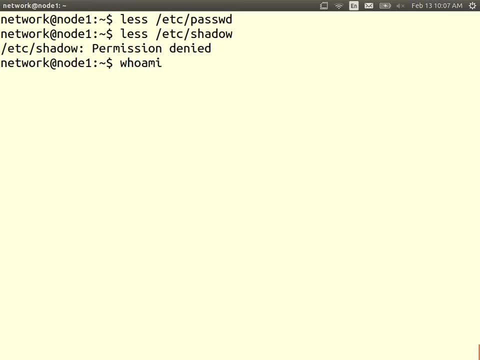 which is network. I'm currently logged in as user called network, So the subject called network is trying to access. read the file shadow. The access control function is checking before they allow them to do And it checks and it finds out no. 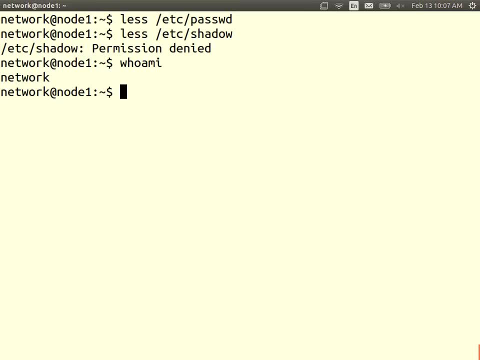 they don't have the access right to read that file. So our operating system has this access control function built in. How can we see the matrix or the access control list? How do I know which files I can and cannot access? LS minus L. 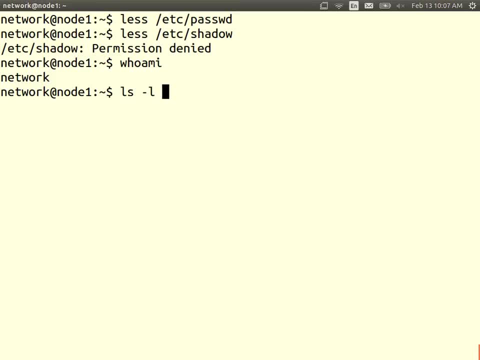 If we list a file, there's different ways to do it. LS minus L just lists the file information in long format and it tells us some information about the permissions. So this is the file and it tells us, and we'll recap these nine characters: tell us in short form: 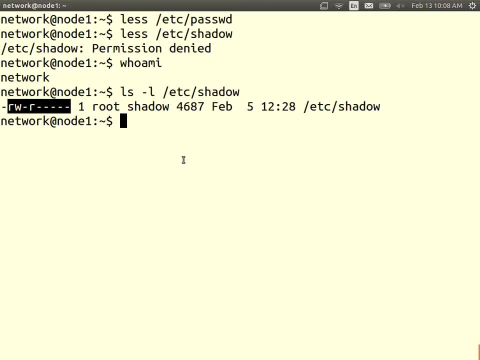 the permissions on this file. For this file, the user that owns the file is called root, That's the owner of the file. That user has the permissions of read and write, but they do not have execute permissions. That's how we interpret those three characters. 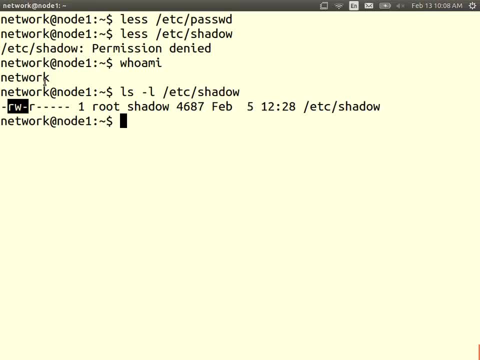 RW dash means R for read, W for write. The third character should be X for execute. If there's no character there, just a dash, it means we don't have that permission. So the root user. so the root user has read-write permissions on this file. 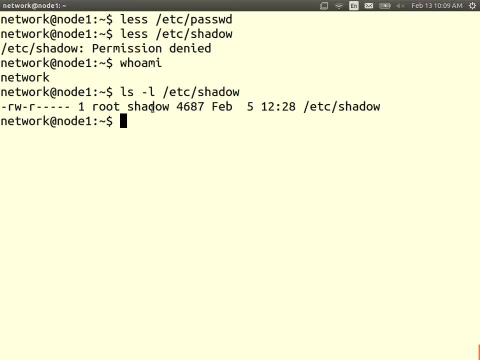 But there's a separate classification of users. There's also a group of users. The group is called shadow. Anyone inside that group has these permissions. Anyone inside that group has the permission to read the file but not write or execute, And anyone outside of that group. 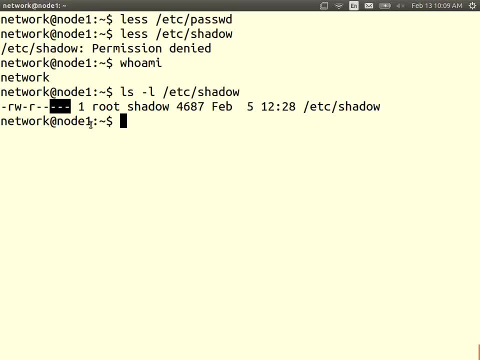 has no permissions on that file. The network user is in these groups. They are not in the shadow group. So the network user is not the owner. They are not in this group. Therefore, they're one of the other users, The other set of users. 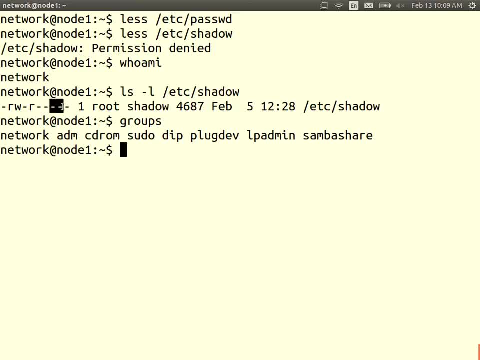 So that the permissions that the network user has on that file is defined by this setting, which means they have no permissions, They cannot read, they cannot write and they cannot execute. That's why when we try to look at the file, it says permission denied. 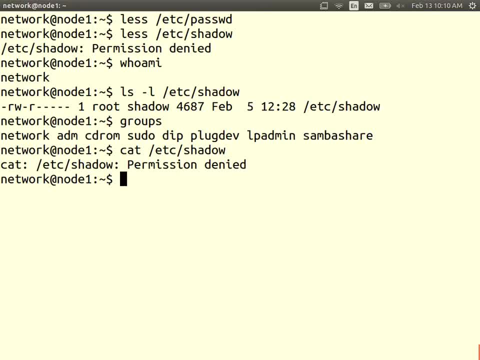 So the access control function uses this information. So somewhere it's stored on the file system And it checks the permissions. And when someone tries to open the file to read it, the access control function of the operating system does the check and, in this case, determines they don't have access. 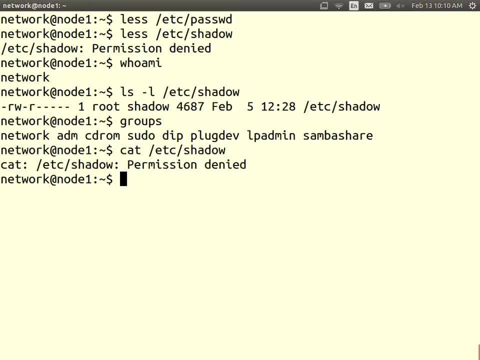 So that's an example of the access control in operation. Is this system discretionary, Discretionary access control- What's discretionary access control mean? I know we haven't looked at the other two, but what's the discretionary part? Why do we call it discretionary? 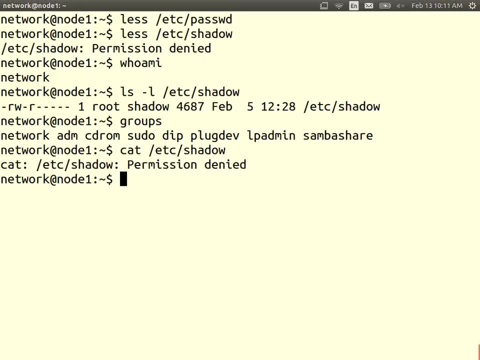 What's it mean? They mention user and resource. No, not Think of the word discretionary. Discretionary Or the users have some discretion to do something. Discretionary means that the users can choose to change the permissions. They have the discretion to make changes really. 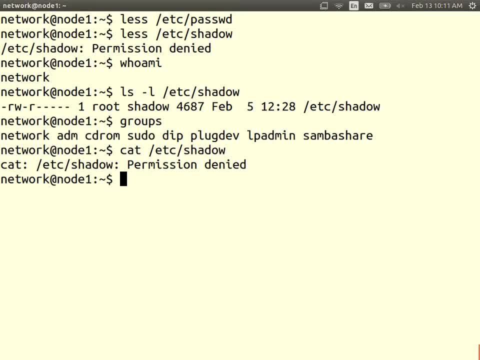 So in other systems we'll see later that the users cannot change them Once the permissions are set. so once the initial permissions are set the users cannot change that. But in a discretionary access control a user has the ability to change these permissions. 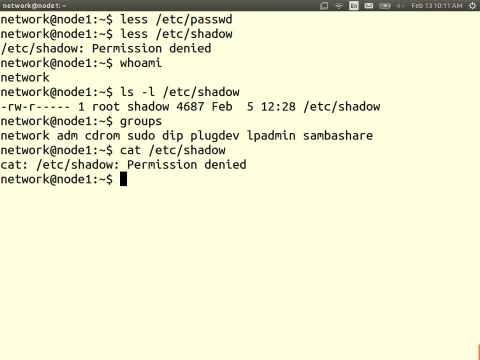 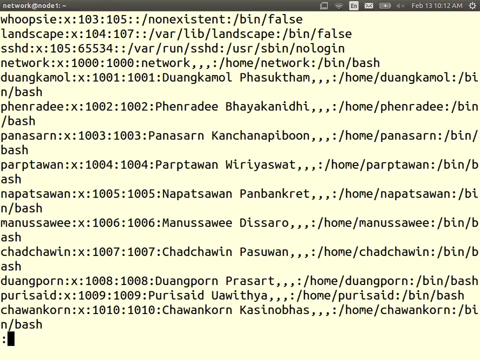 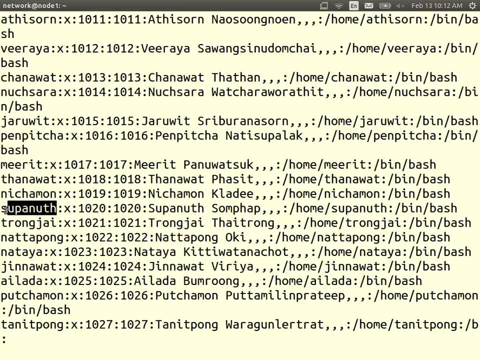 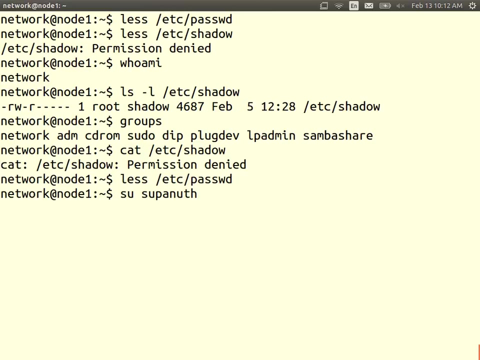 especially of the files that they own, And we can do this in this system. Let's switch to a different user. Any volunteers? Who's going to volunteer? Okay, thank you. Can you tell me your password? I want to switch to this user. 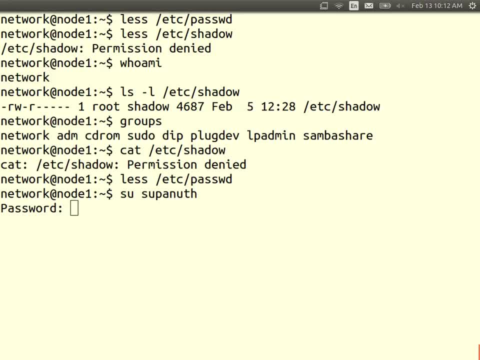 but I need his password. You want to guess? Brute force Failed. Our authentication is not working. is working in that if you type the wrong password. So this is back to our previous topic. Note when I typed in the password. 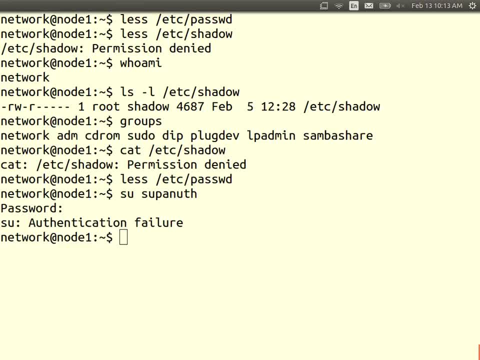 and I'll do it again. I think we've seen this, but we'll do it again. All right, It prompts me for the password. I type in a password. I know it's the wrong password. I press Enter now. It takes several seconds before it returns me to. 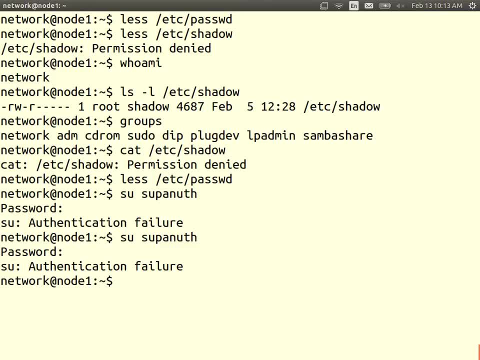 A. it says there's a failure. It doesn't say wrong password or even wrong username, but in this case it's just saying it didn't work And, importantly, there was a delay. So when I pressed Enter, until when it returned me to try again. 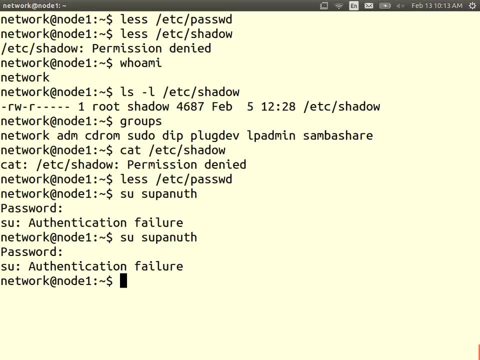 there was a delay of several seconds. It doesn't take my computer long to check. It takes microseconds to check. So the delay is some arbitrary or some introduced delay to make it slow for brute force attempts. It means someone cannot try many passwords. 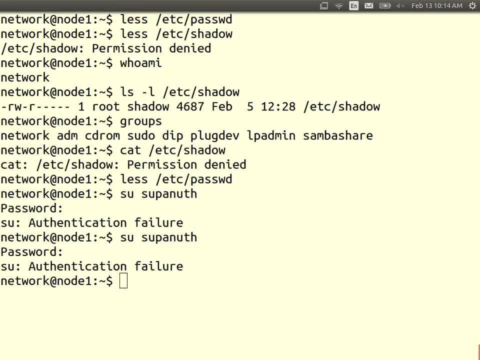 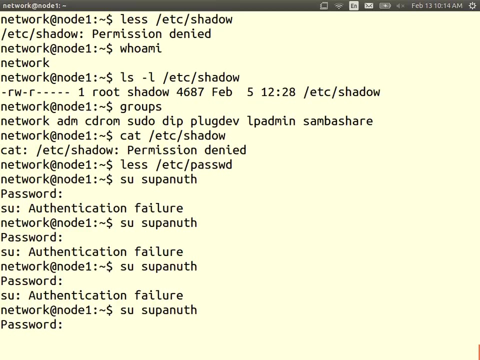 I need to remember or try and guess the password And try again. If I keep trying, do you think it will lock me out? No, On this system it. I think I've done it again. If you keep trying, it will just allow you to make multiple attempts by default. 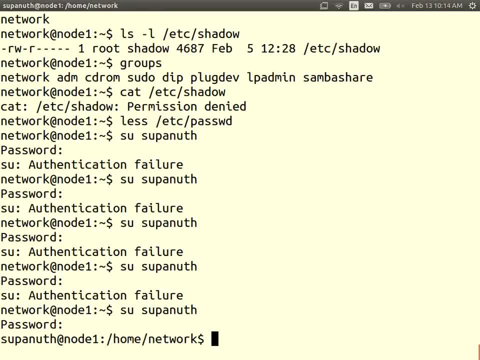 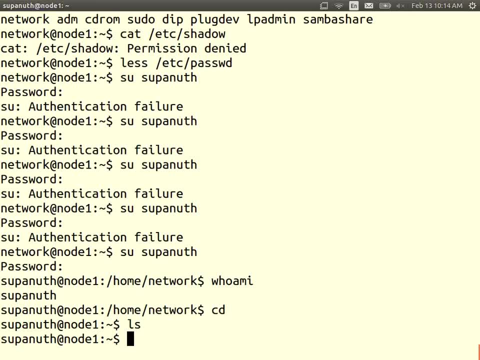 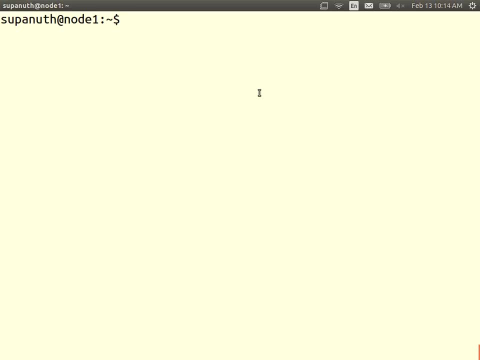 Maybe I don't know the password. Okay, We're there, So we're logged in as a new user. now, Okay, Let's create a file. I made a mistake, didn't I? So in this case, our user has permissions on this file. 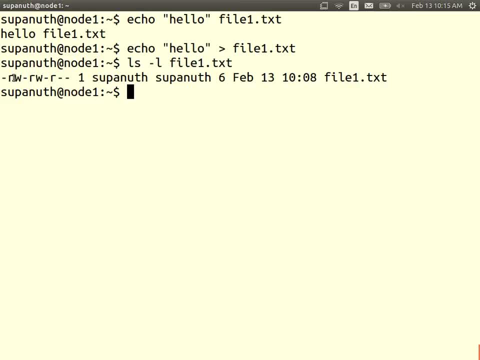 which are read-write. The user that owns it has read-write permissions. The group- anyone in that group- has also read-write permissions. Anyone else has read permissions. That's how we interpret. Anyone else? It turns out by default. no one else is in this group other than the user. 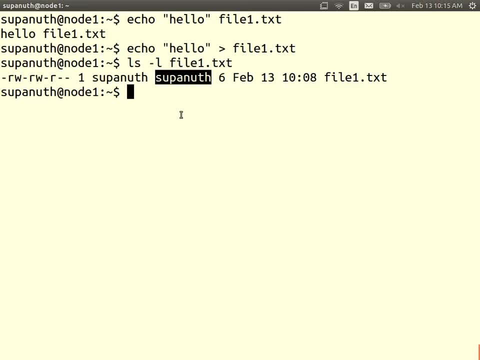 So the default permissions say that for this file the user is allowed to read and write. Everyone else is allowed to read the file only. They cannot modify. So they're the default permissions. We can change permissions. How do we change permissions? Question. 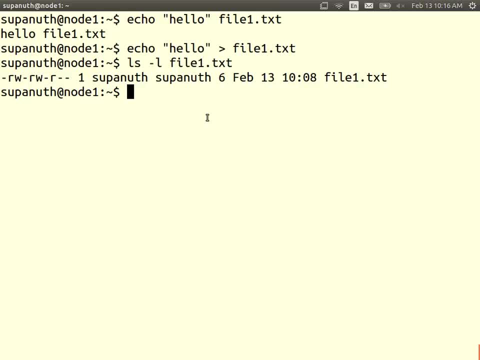 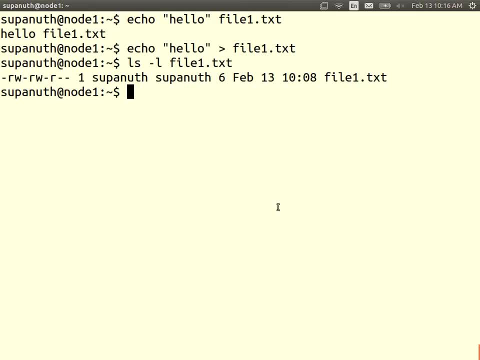 CHMOD, CHMOD, CHMOD- possibilities. Well, let's change the permissions and see some things that we can do. We may see the role of ownership. So let's change the permissions and we'll make some different changes and see what can happen. 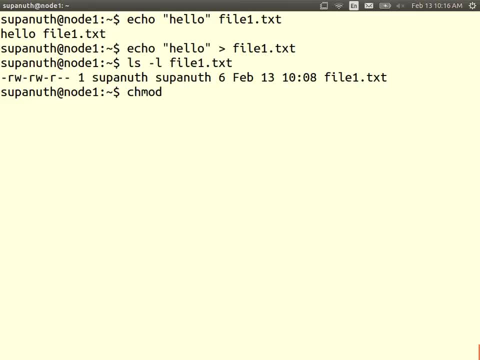 We can change permissions with this command, Change the mode at which people can access, So an access write or an access mode, And we can say, for example, others cannot read the file, Subtract them the write or revoke the read permissions of that file. 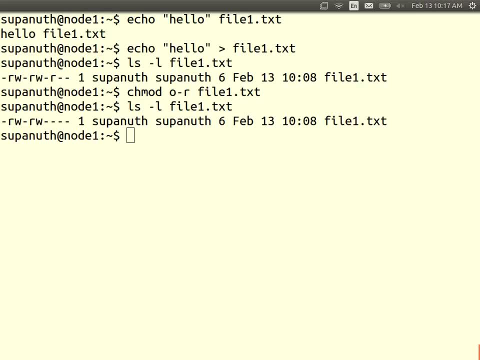 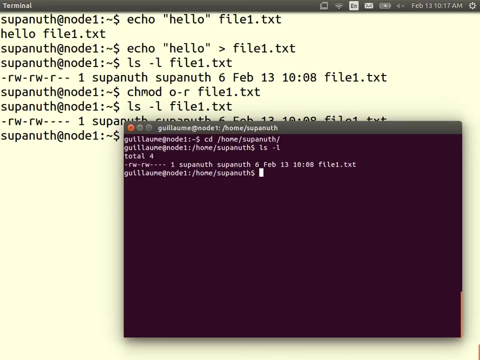 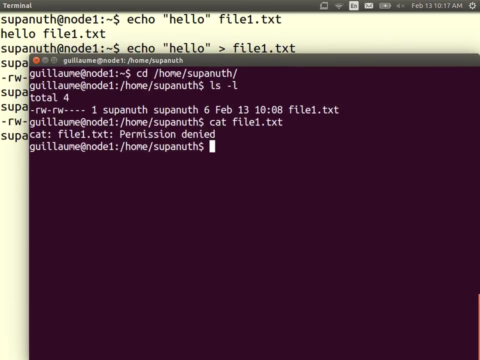 And we'll bring up another user And our other user. I'm logged in as another user. now can they read the file? Let's try. Permission denied. So my alternative user cannot read the file and if we change the permissions back others. 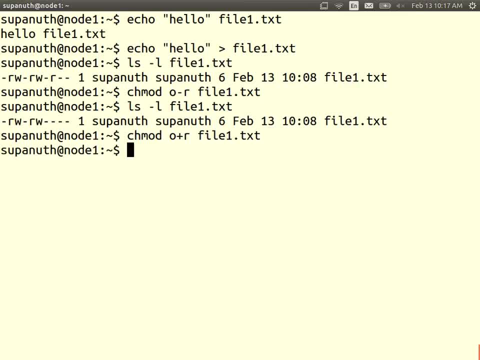 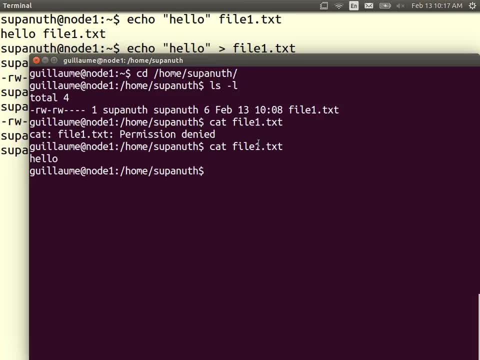 can read the file. We now can read the file. So that's just changing the mode of the file, which is this discretionary part of discretionary access control. The users have some ability to modify the permissions. What do you want to do? Remove the permissions for everything. 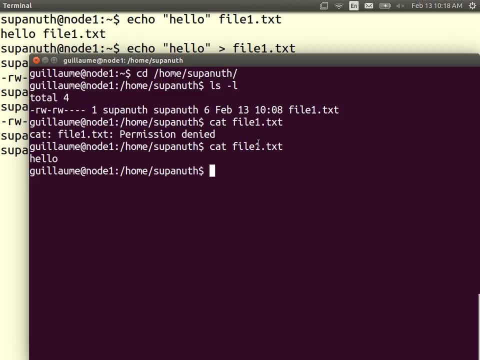 Let's see what we can and cannot do. Can this user Change the permissions? Let's try No. So normally the user that owns the file has the ability to change the permissions. In this case, our user has the ability to read the file, but they don't have the ability. 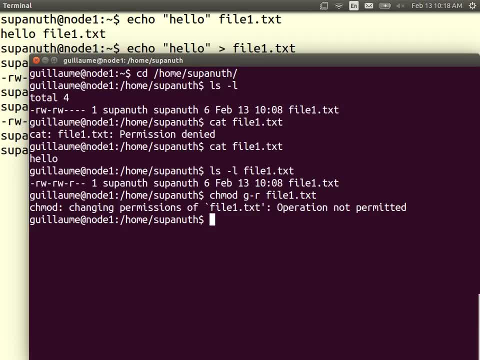 or the discretion to change the permissions on that file. So that's usually the right thing to do. So that's the right thing to do. So that's the right thing to do. So that's the role of the owner, why we often specify the owner. 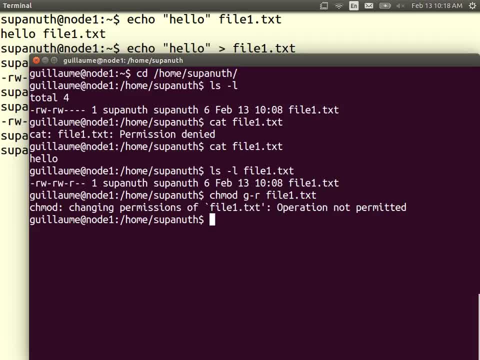 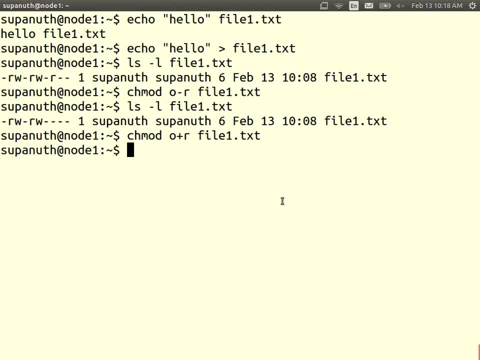 The owner can change permissions, but other users, even if they can read the file, cannot change the permissions on that file. Everyone cannot do anything. A for all users. subtract or revoke the permissions of read, write and execute. A for all users. subtract or revoke the permissions of read, write and execute. 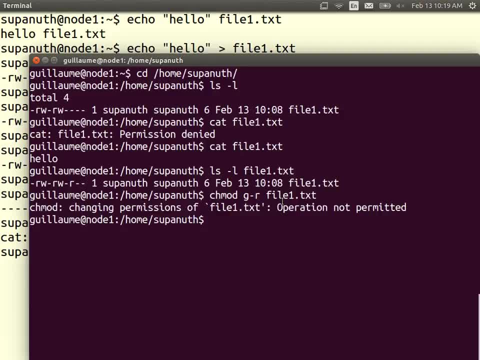 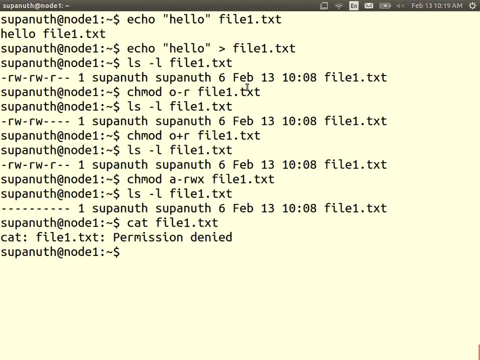 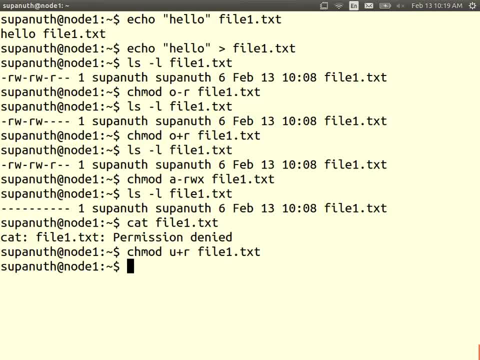 That's a problem. That's a problem, But the owner can still change the permissions. So there's this fourth access right. we have here ownership. So now, previously the owner could not do anything with the file, but they're still allowed to change the permissions. 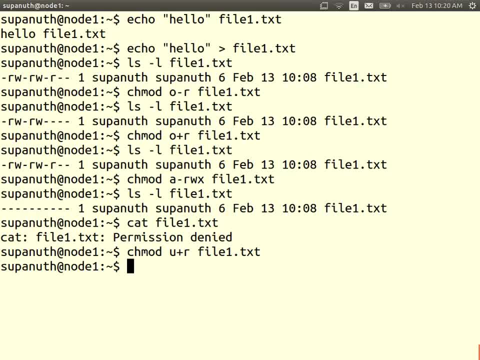 So we change the permissions back so that we can now read the file. So that's the normal, the normal, the normal case in that a user can change permissions if they own the file. so think of four access rights so far: ownership, read, write and execute. and 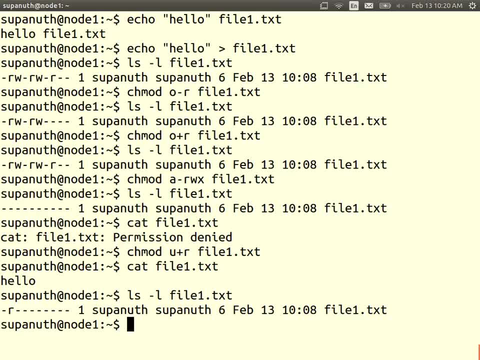 that's what's default on a on a Linux system. on other systems they may have other access rights and different meanings. so what we're going to do, your next homework task will involve just looking at permissions, and that's where you need to use one of these virtual network nodes so that you all have the